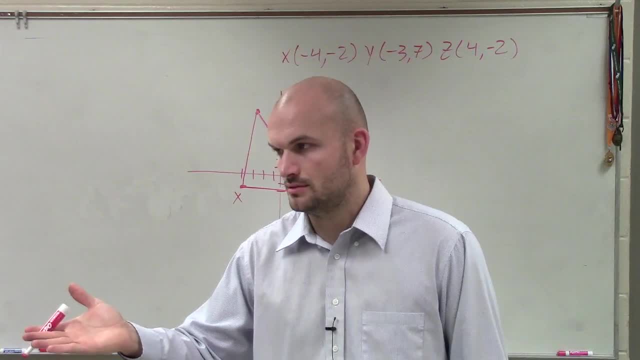 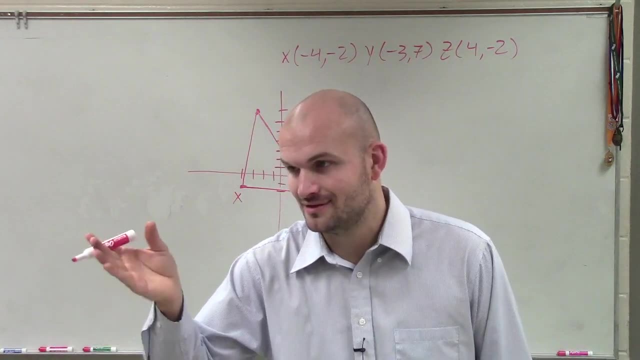 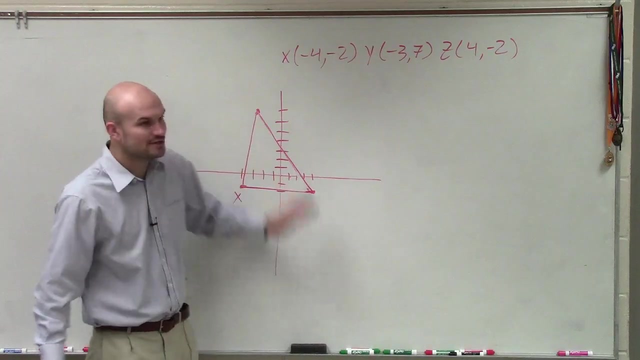 how many sides are equal? All, No, Equilateral is all three, Isosceles is two And, Angel, if it's scalene, how many sides are equal? None, Thank you, Angel, You have a really high voice. Yes, It's just zero, right? So how are we going to determine the length? 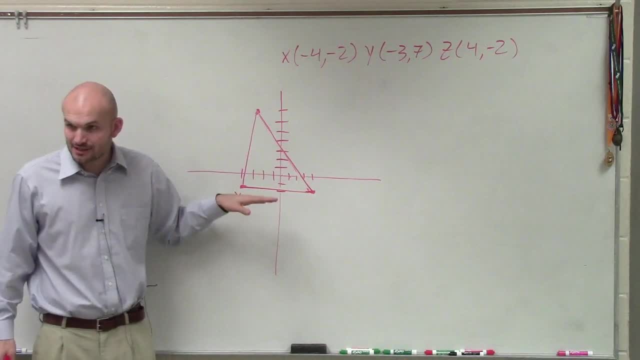 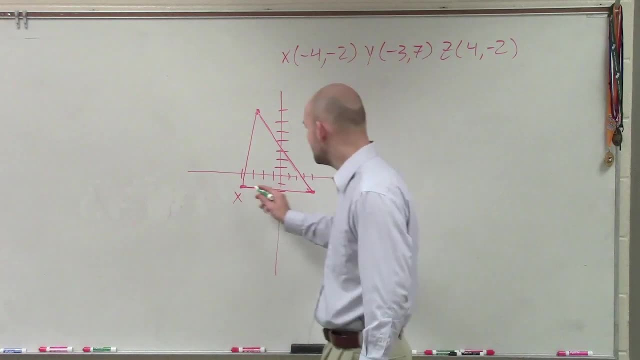 Well, this one, you guys can see this is a horizontal line, right. It's not changing up or down. So this one's fairly easy. What we can do for this one, Mario, is just count the number of units. 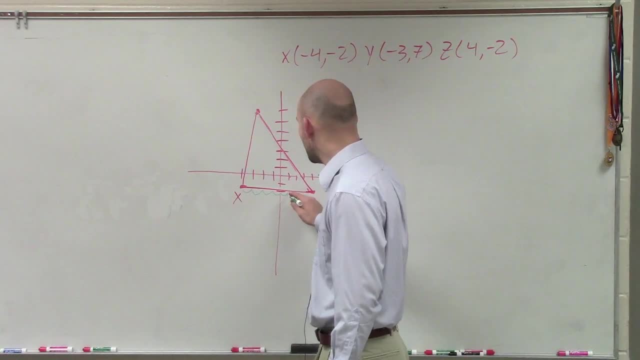 1., 2., 3., 4., 5., 6., 7., 8., So that one has a length of 8.. But now we need to determine what is the length of the other two sides. Well, guys, you can't just estimate and say: well, this is going. 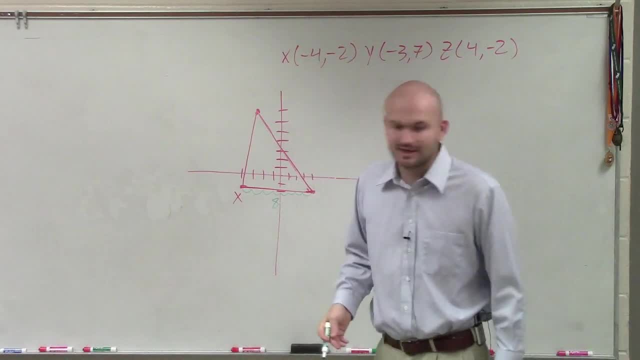 to be 1,, 2,, 3, 4.. It doesn't work like that. All right, That would be an estimation. We're trying to find the exact value. So does anybody remember a formula that we did between two? 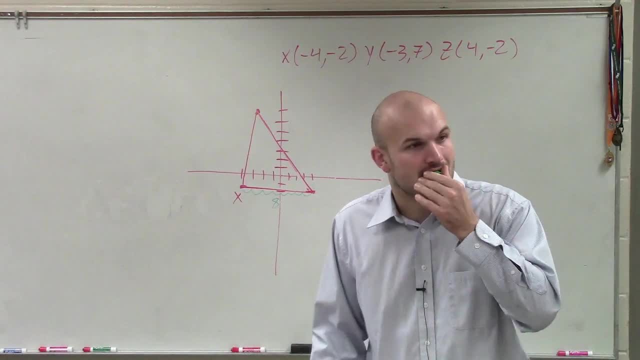 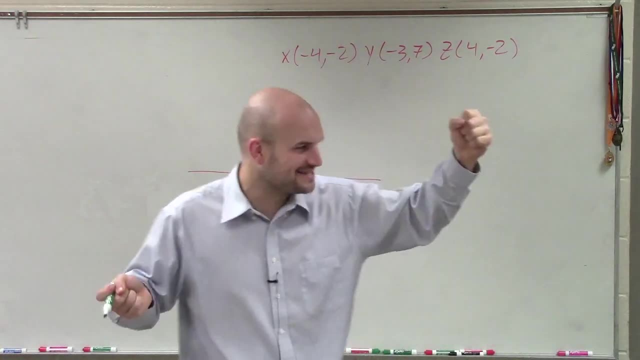 points to find the distance. Yes, Zach Slope. Well, the slope form is going to tell us, yes, the rate of change, But I want to find the distance. What was that formula that had distance? And it was a formula. Yes, 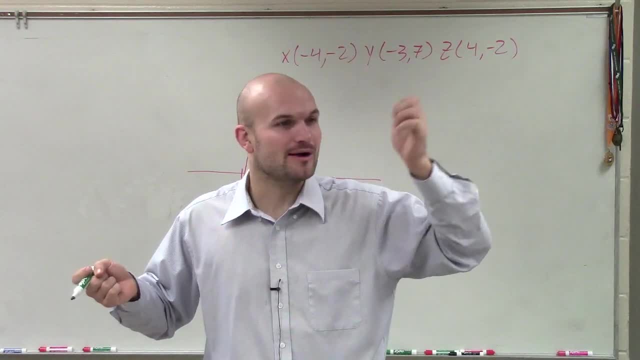 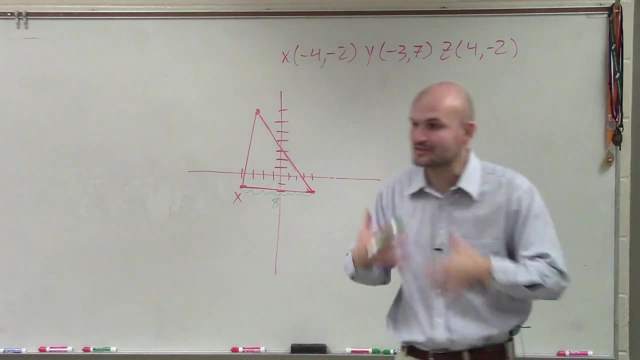 Zach, Distance formula 1. Right, Well, what the name of it, though, was The distance formula right? So that was something that we learned beginning our class, And I said, ladies and gentlemen, we're going to constantly be going back to this right, Hence why I said you really need to. 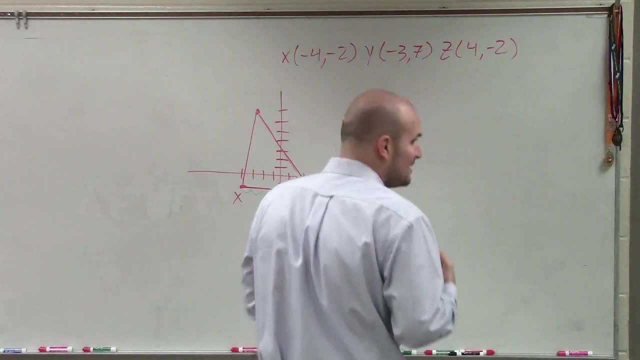 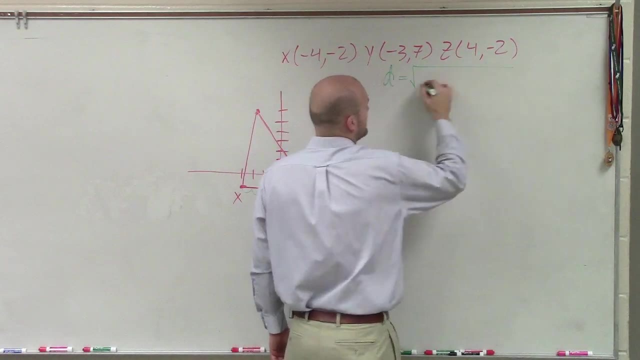 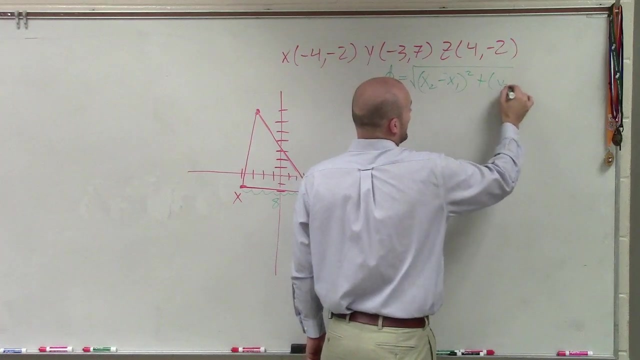 make sure you know this formula because it's going to keep on coming back And you're not always going to have it available to you. So, yes, the distance formula And the way the distance formula goes, is the square root of x2 minus x1 squared, plus y2 minus y1 squared. 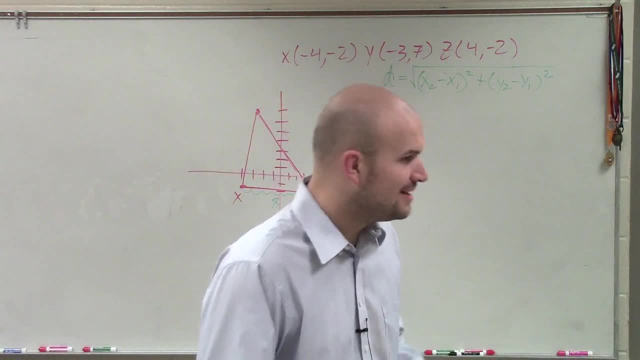 We have to know the distance formula. We are going to continue using this formula. It is going to pop up in questions And it's not going to be what I'm. I'm not going to say find the distance between two points, but I'm going to ask you questions and you're. 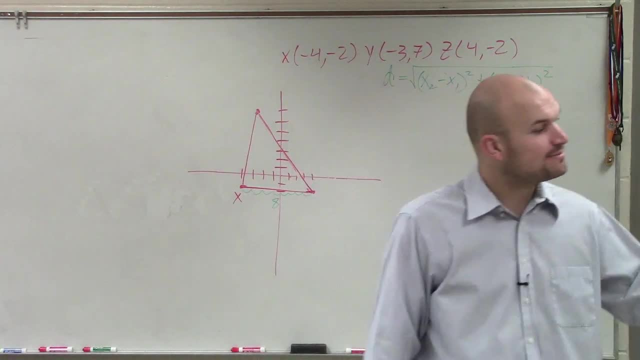 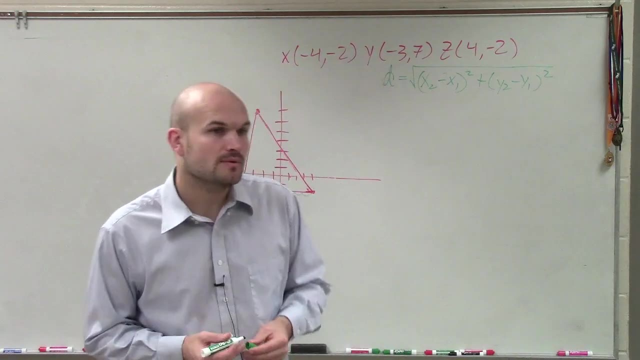 going to have to know how to find the distance between those two points, to ask my original question that I'm asking. All right, so this is going to be embedded now in the rest of this curriculum. so, Damon, if you wrote down the wrong problem, what I'd like you to still do is go ahead and write this one down as well. 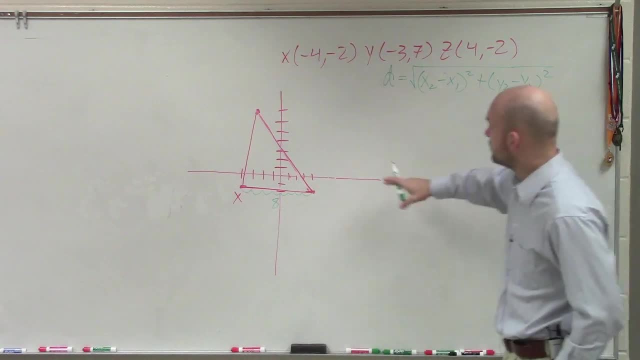 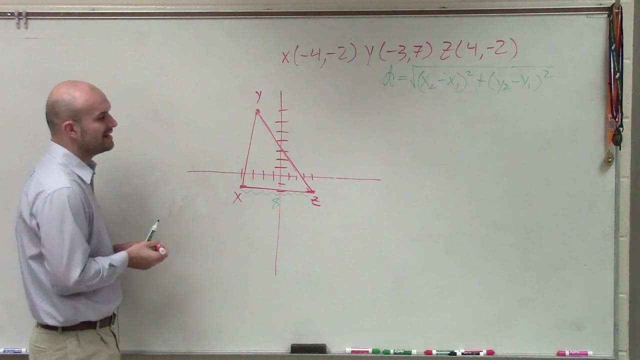 Okay, so now what we're going to do is we need to find the distance. well, I didn't label these. that's x, that was y and that z. all right, So we already know the distance between x, x and z. let's find the distance between x and y. 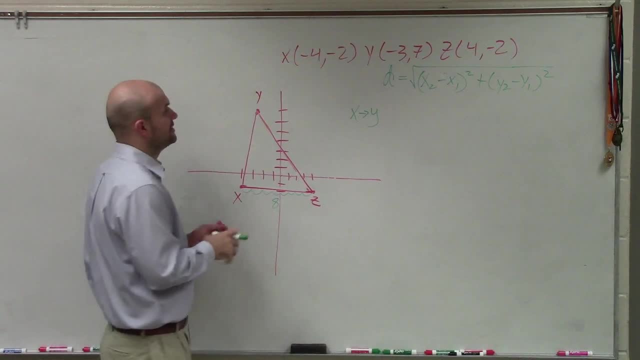 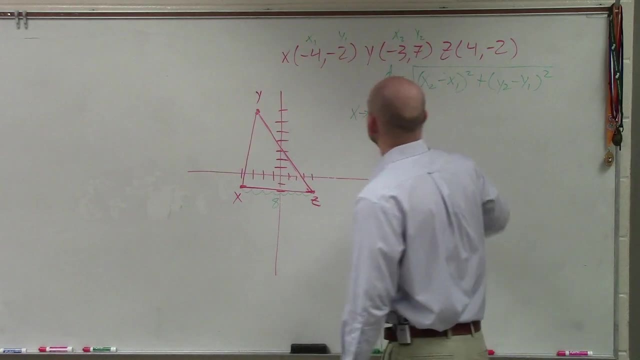 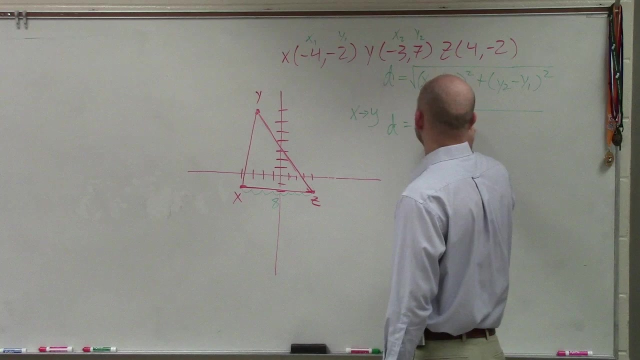 So let's find this distance between x- y. well, what I can do is then label them. I'll call that x 1, I'll call that y 1 y, I'll call that x 2 and I'll call that y 2. So I say the distance between x to y is going to equal to x 2, which would be negative- 3 minus negative. 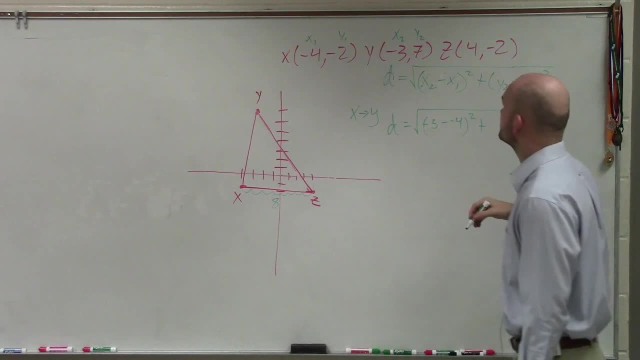 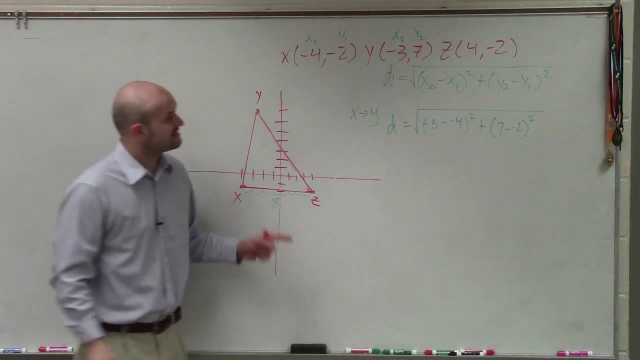 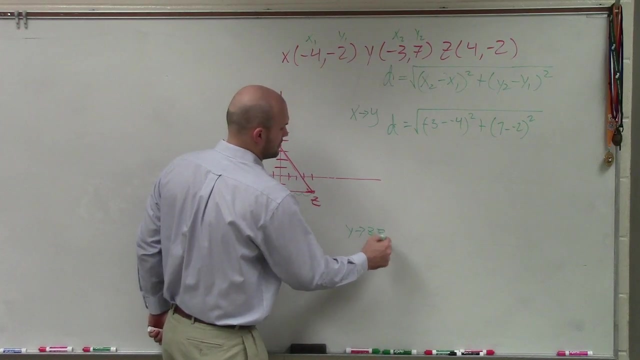 4 squared plus 7, minus a negative 2 squared. and Then let's find the distance. before I Even simplify this, let's find the distance between y z, Because, remember, guys, we don't even need to actually find everything, we don't need to do so much of the work. 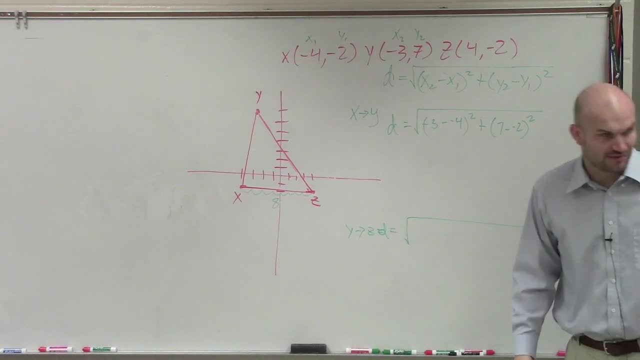 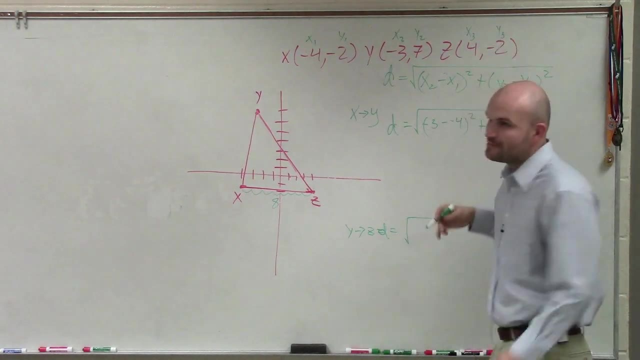 That all you guys are doing. now I'm going to maybe be a little confusing with you. if this is x 1, that's x 2. I'll call this x 3. you don't have to. But remember, when you're finding the distance, all you're doing is you're finding the difference between the two x coordinates. 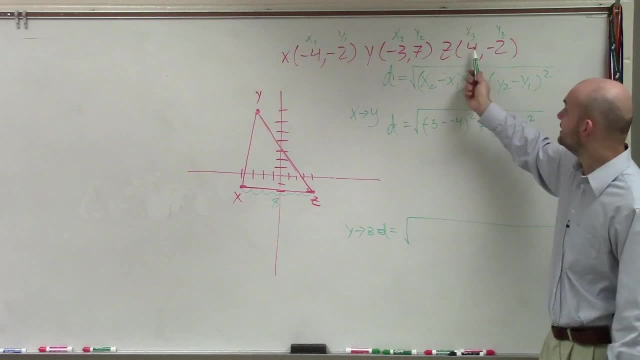 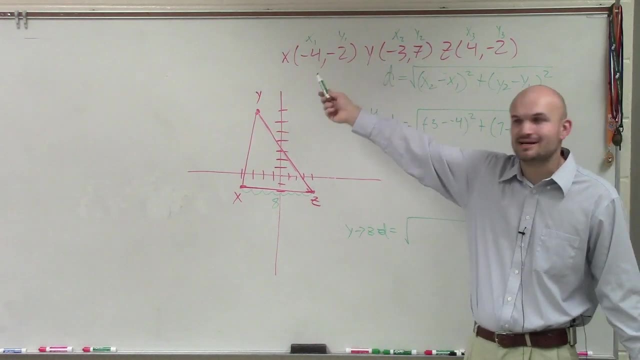 All right. so in this case I want to find y to z. I just need to find the difference between these two. so I'm just going to do x 3 minus x 2. It's the same thing as x 2 minus x 1, all right. 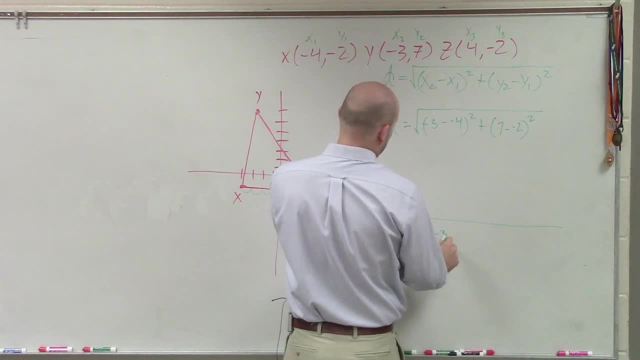 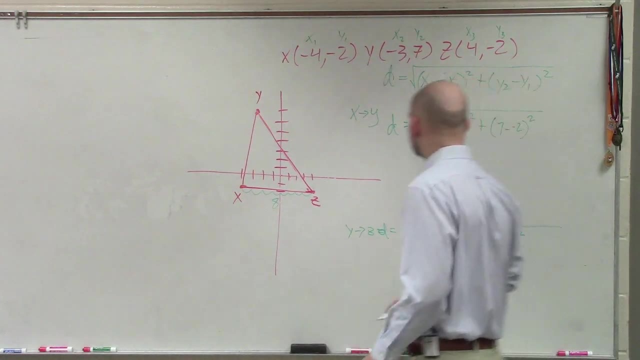 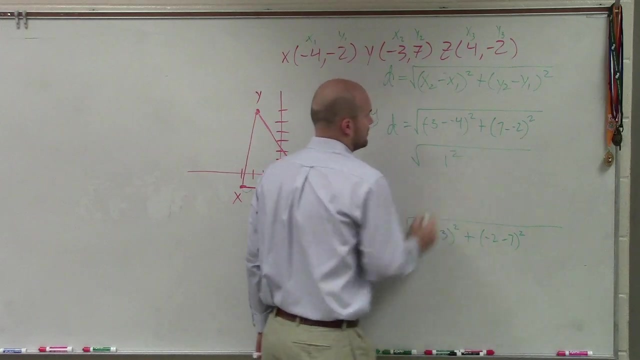 So therefore, I'll have 4 minus a negative 3 squared, Plus negative 2 minus 7 squared, so negative 3 minus a negative 4, that's going to be square root of 1 squared, and And 7 minus negative 2, that would be plus 9 squared.